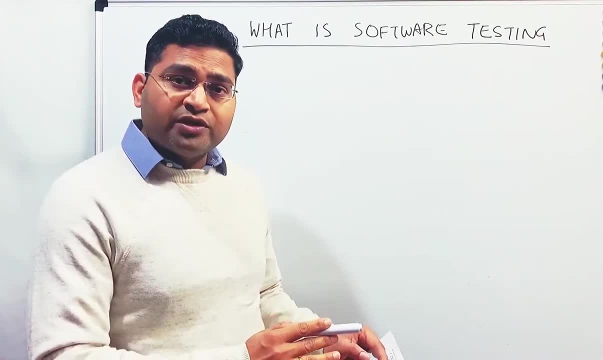 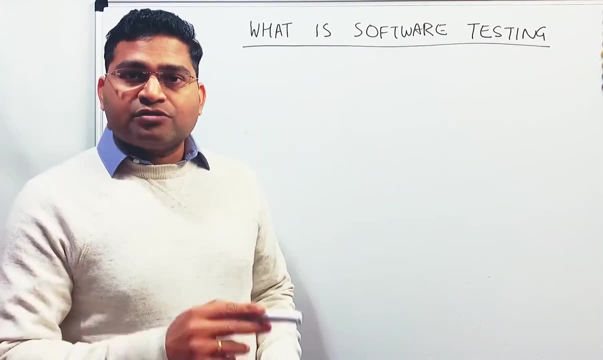 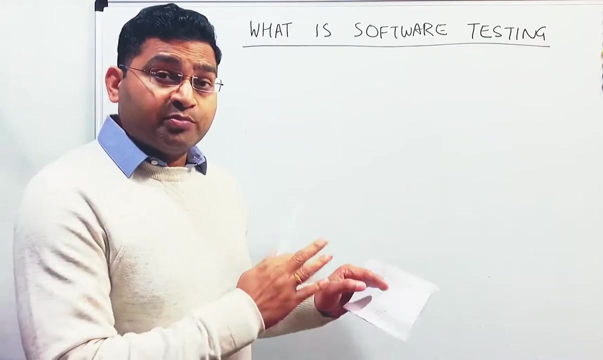 testing job. you need to understand basically what is software testing before you can learn any other concepts. All right, so first thing, we need to understand what is software testing. Watch this video till end so that you do not miss any of the key concepts that I'm going to explain. 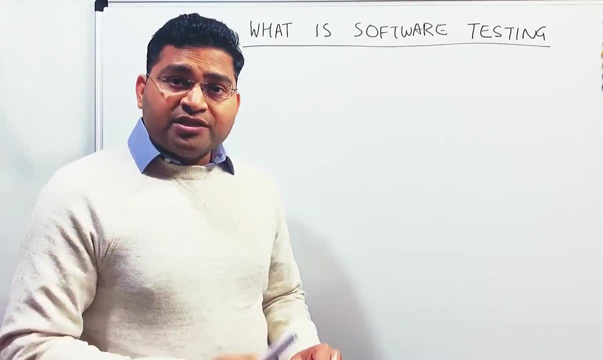 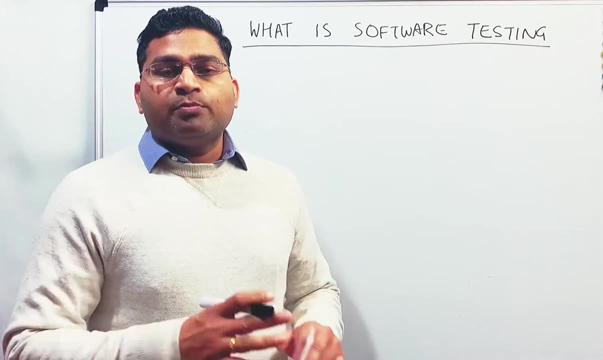 in this particular tutorial. Before we understand software testing, let's first understand what is testing in general sense. Say, for example, you go into the market, you buy any product, you take it back home As soon as say, for example, it is an electronic appliance. 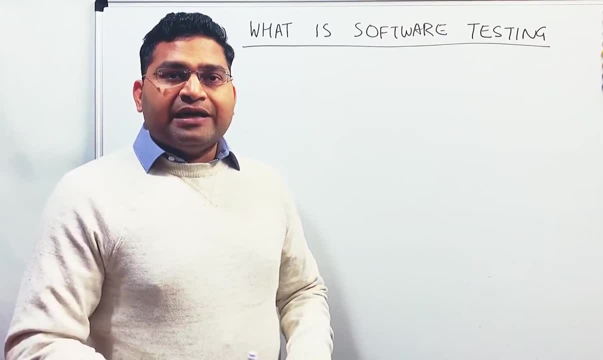 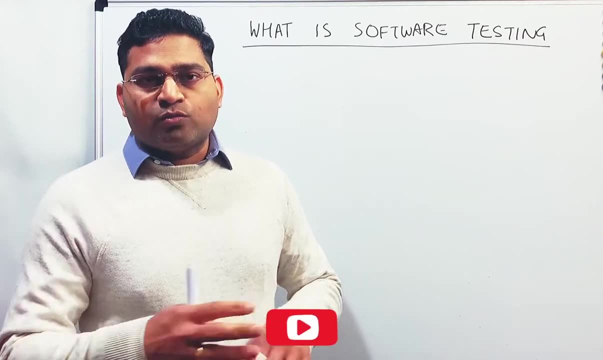 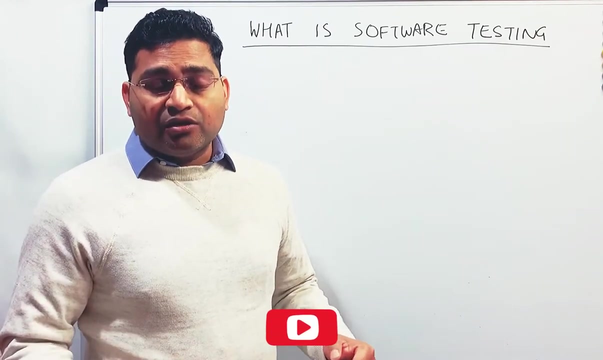 or any kitchen appliance. you plug it in and it you know it doesn't work. It doesn't turn on or if it turns on, it doesn't function properly. What is your feeling in that particular case? You are really annoyed, or we get really annoyed with the company or the product you know. 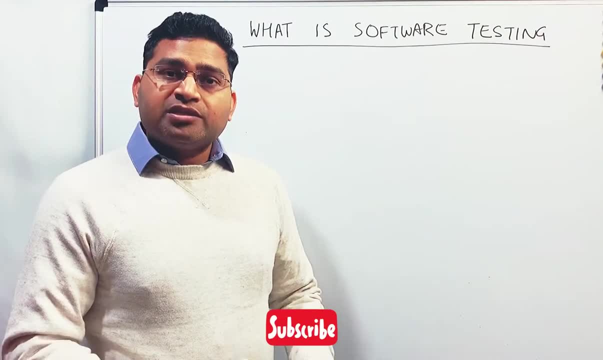 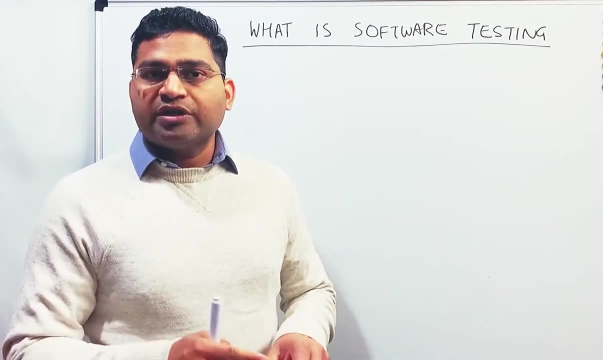 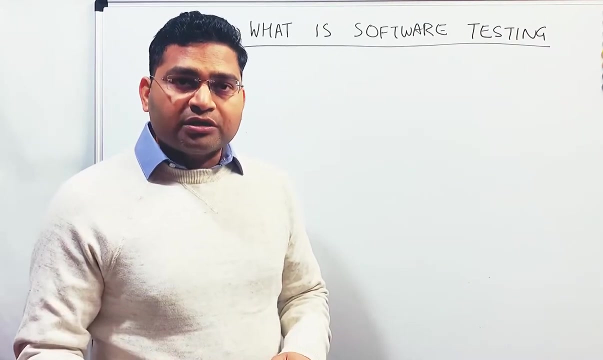 the company that has provided that product And we question the quality assurance or the quality criteria That company has for their product line. right Now, how do the companies ensure that they are delivering the quality product? It is through the testing right, So it doesn't matter whether you 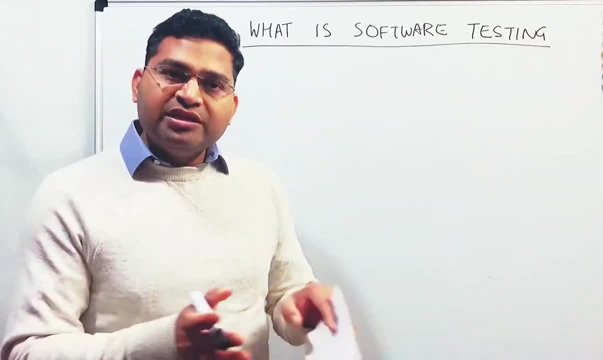 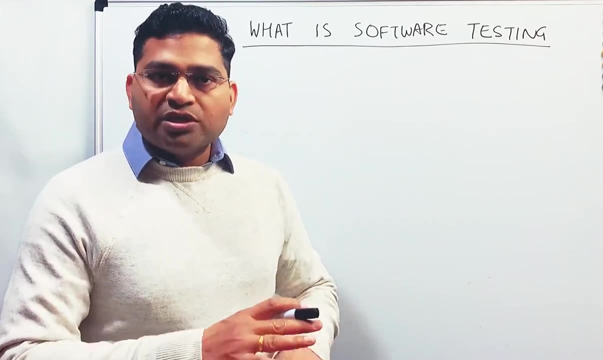 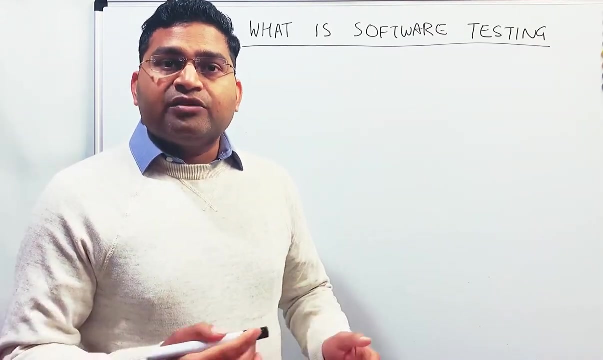 are buying a car, you are buying any electronic appliances or anything else. There is always a level of testing involved in any of the product that goes into the market that you buy. All right. So even if you are, you know, taking any of the services- say, for example, you are, you know, opting for any services- 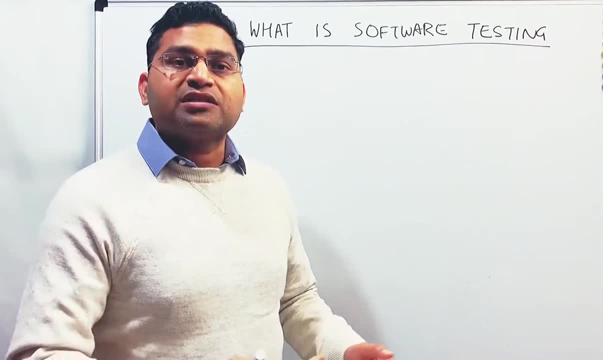 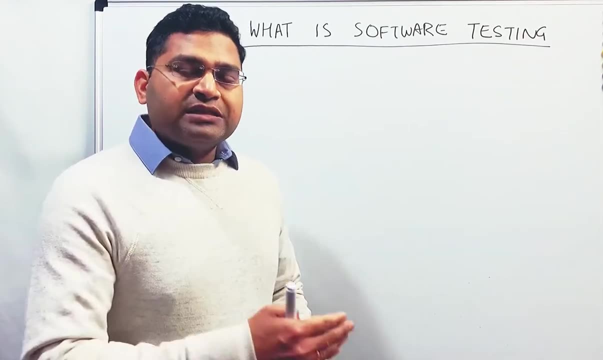 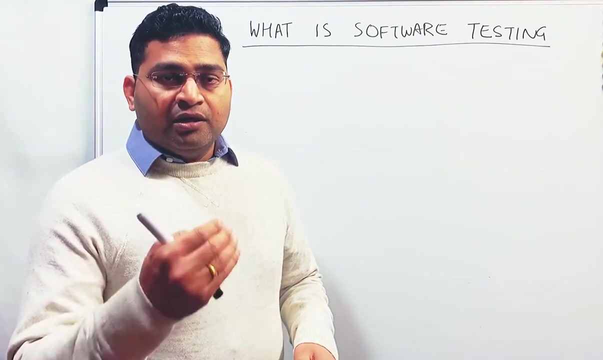 you also consider the quality of the service right, How the customer services. So quality is everywhere, whether it's a service or product. Now, when it comes to products, it is basically ensured through a defined or predefined process of testing. So that is, in general, what testing is. 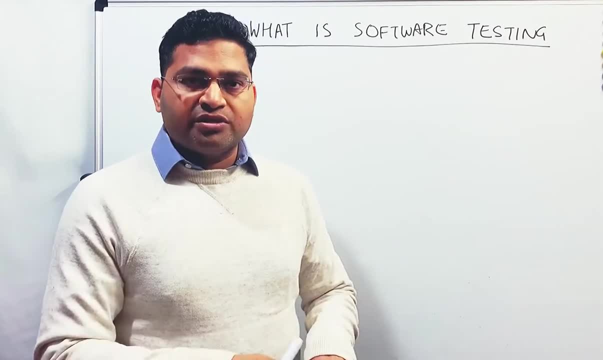 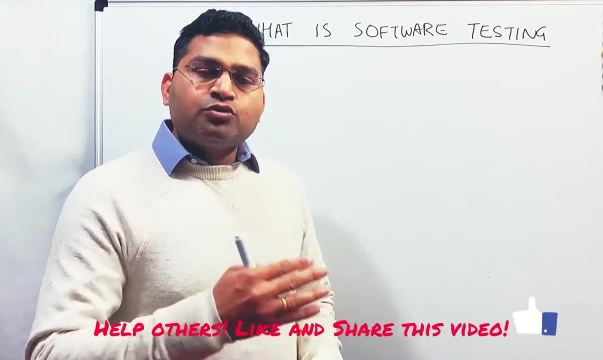 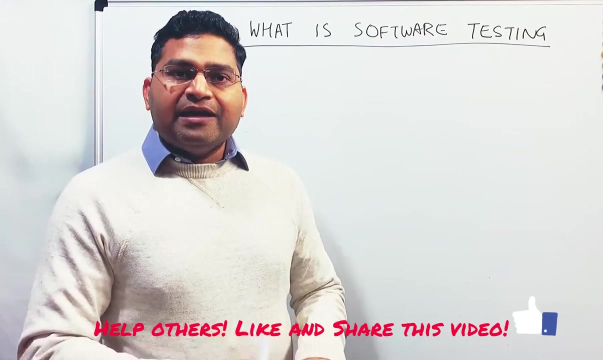 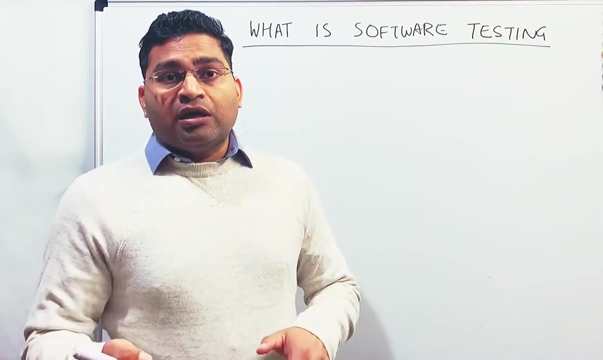 If we talk about the product or any other product, it is basically a predefined process of testing. So you know if you are buying an electronic appliance or a food or a beverage or a being. you know some hardware or any other. you know like industries, car manufacturing, electronic manufacturing, et cetera. So they have their own defined processes and tools to ensure that the products that are coming out of the assembly line are being tested properly and work properly before they are, you know, brought into the market and being sold to the consumers and they use it Right Now. when we correlate that to software, when you test the software and you test the software, you will see that the software is tested as it is based on a machine. You will see that there is that machine on the machine. So if you are testing, if you are testing a- 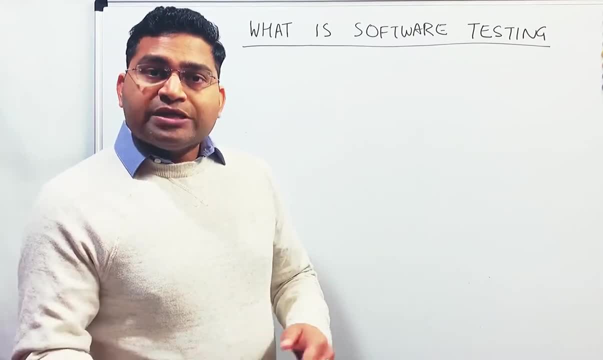 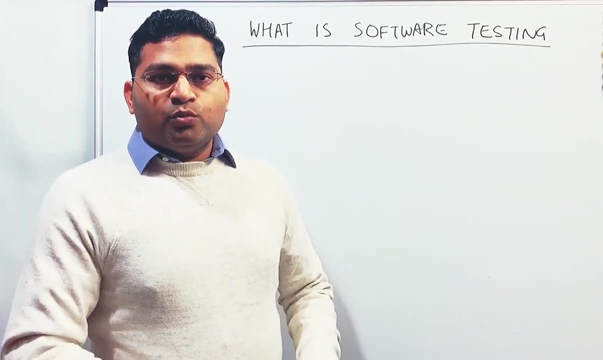 machine, you will see that its own machine, the machine is tested on a machine and you will see that it is based on a machine software. it becomes a software testing. So what exactly is software? Software is any application, say, for example, any website. you take any application which. 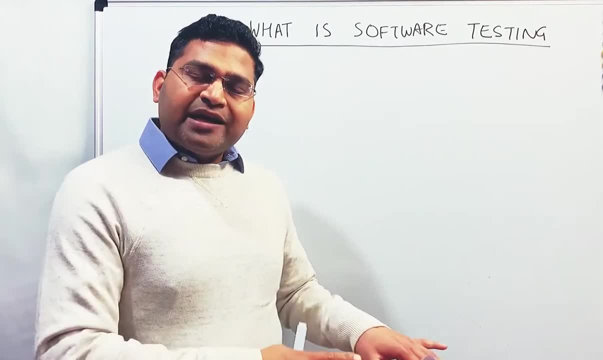 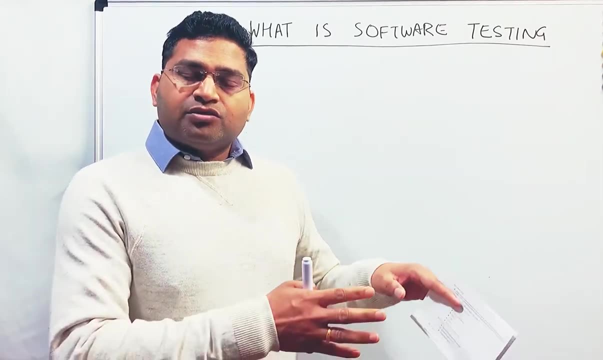 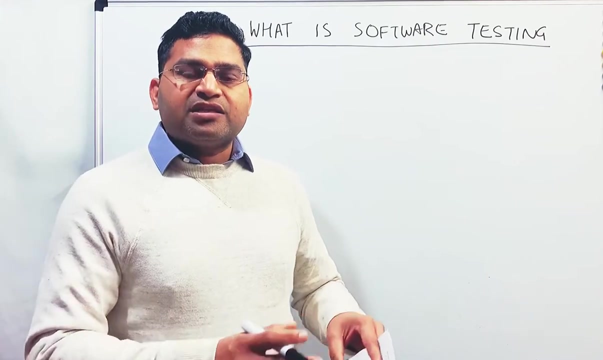 has complex functionality around. you know front-end, back-end web services. So any application which fulfills the business logic is sort of software if it is, you know, like a mobile app or any other application that is available out there over the internet. 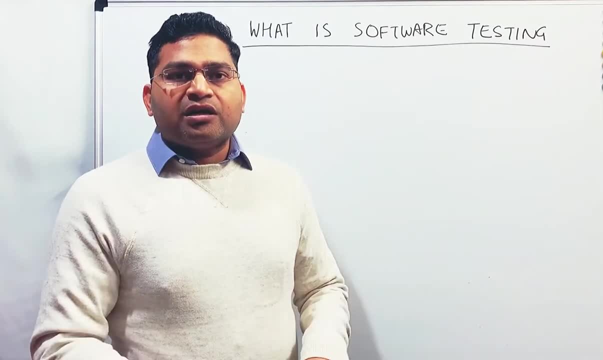 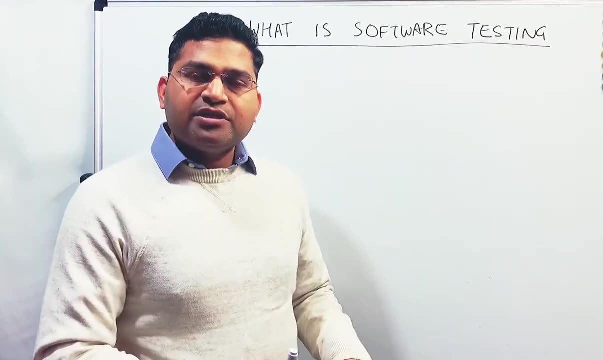 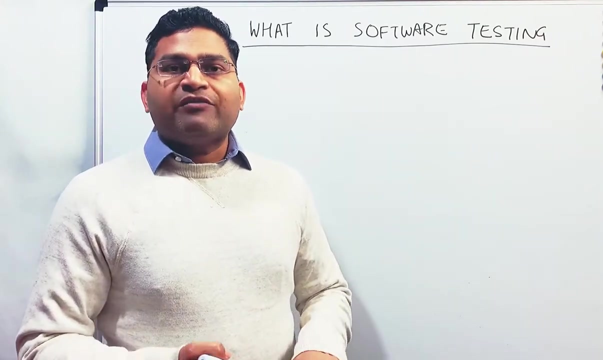 right. So these sort of applications are known as software. So softwares are built into, you know, using many different programming languages, For example, like C, C++, Java. there are n number of programming languages that can be used. Now you have mobile devices, where you have apps. 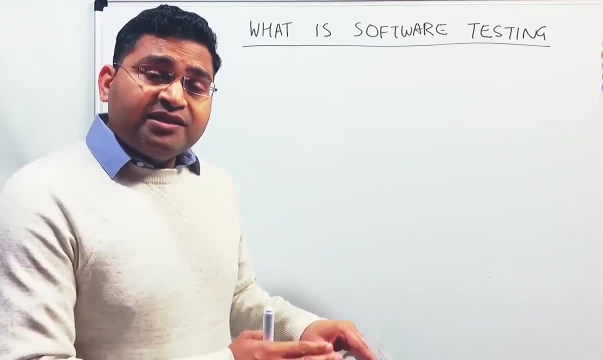 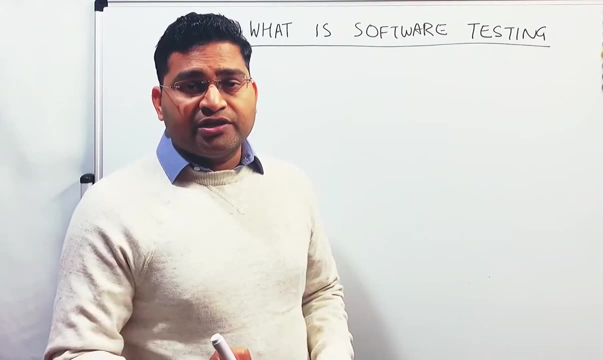 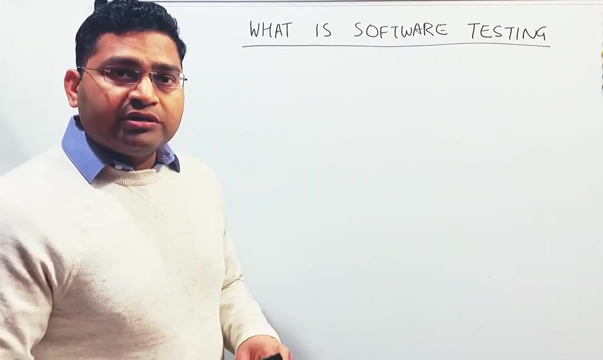 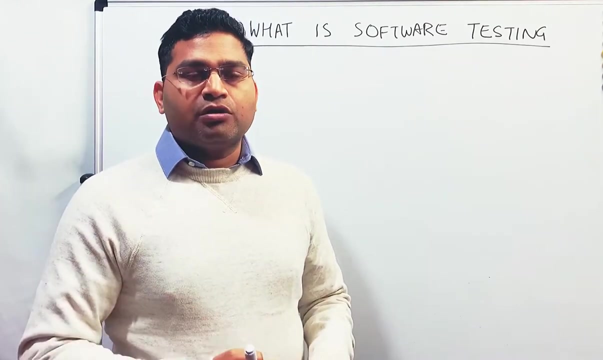 So these are all software. When you are testing these softwares, it is known as software testing. Now, software testing is not a standalone activity. It's a predefined process that you need to follow, from step by step, and ensure that the particular product that you are trying to, you know, put into the market or say for: 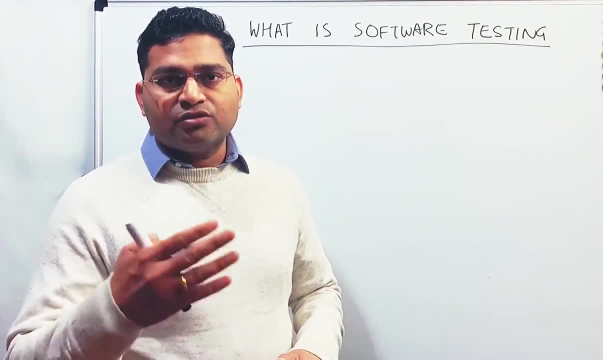 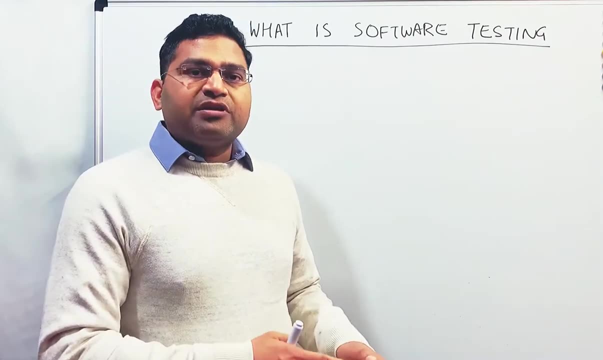 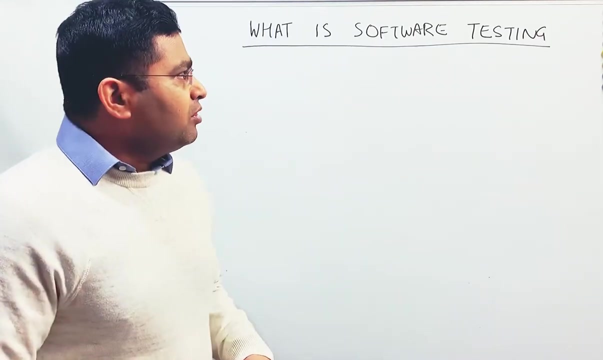 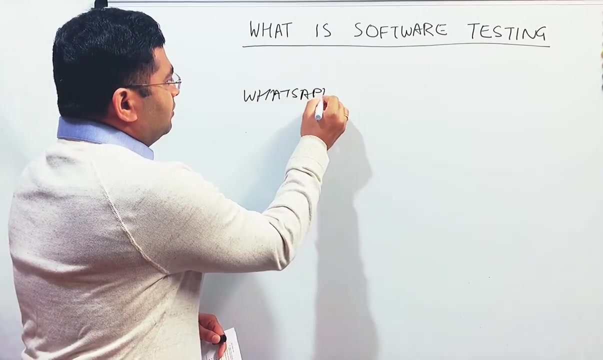 example, an app you want to install or you want to launch it into the app store. prior to launching the app, you want to ensure that whatever functionality that particular app needs to provide to the customers, it works as expected. I take an example of the app. say, for example, WhatsApp- okay, very widely used. 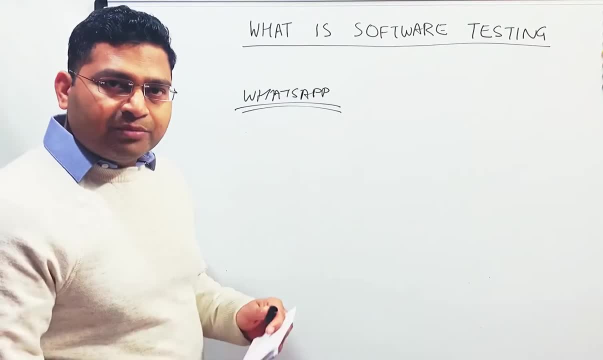 So say, for example, you are building something similar, or you are, you are creating something similar to WhatsApp, So there will be coding done, right? So once the coding is done, there will be code. So once the coding is done, there will be code. 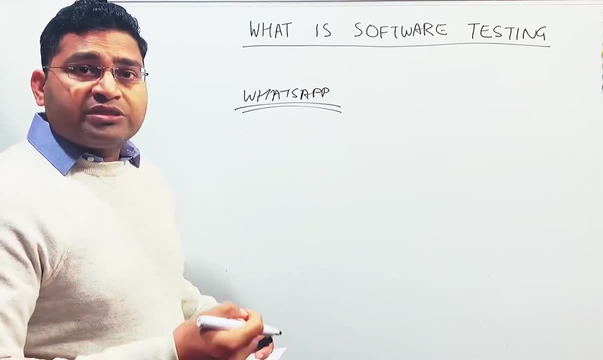 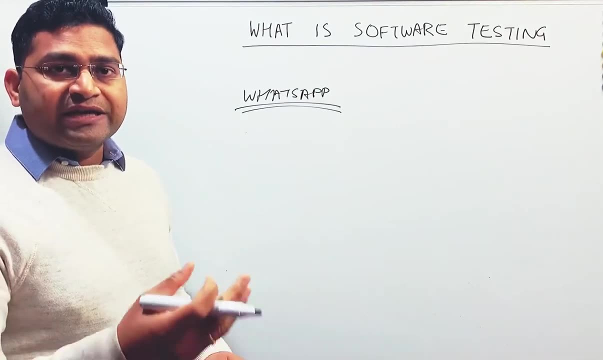 So you should be just added to. for example, I should be able to, you know, send text messages to other people when I, you know, add them in my contact list. right, When I add them in the in the contact list, I should be able to call them. 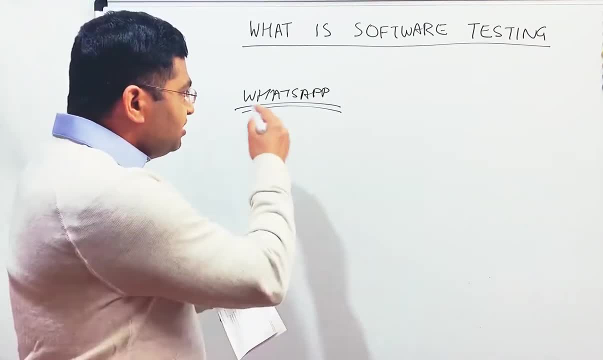 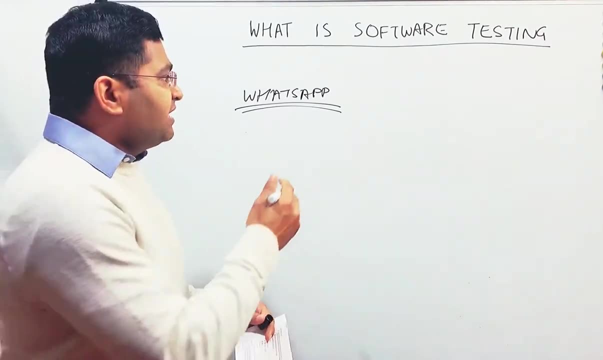 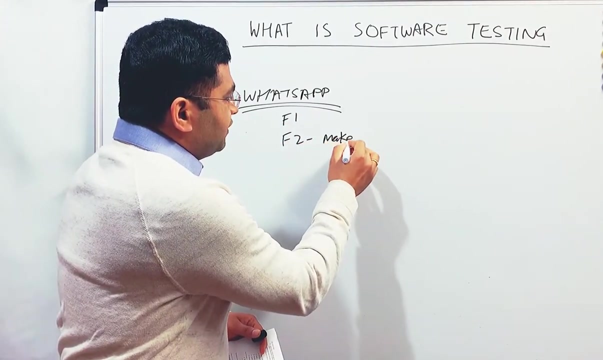 So these are, you know, like some of the features that in the WhatsApp or the app scenario, you will basically test before you actually say that, yes, this functionality, say functionality one, Functionality two is, you know, make call. all right, so I should be able to make call, I should be. 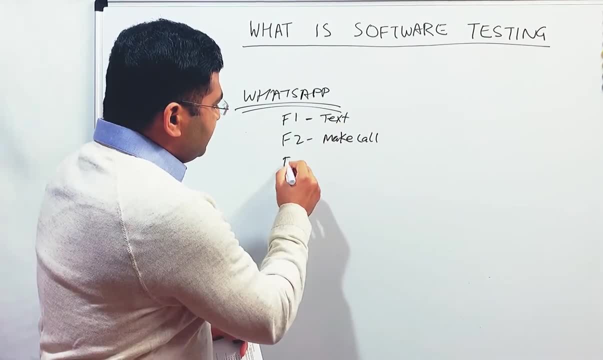 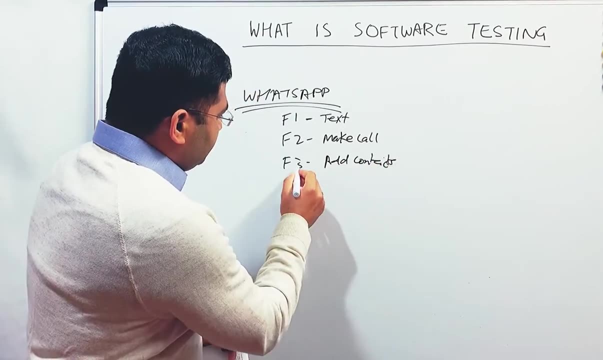 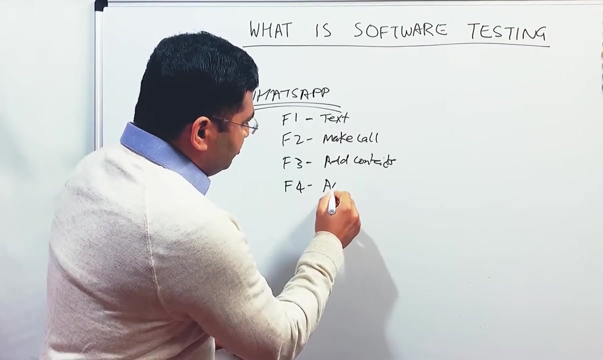 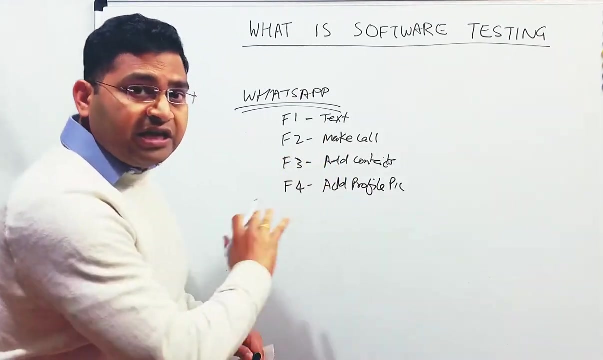 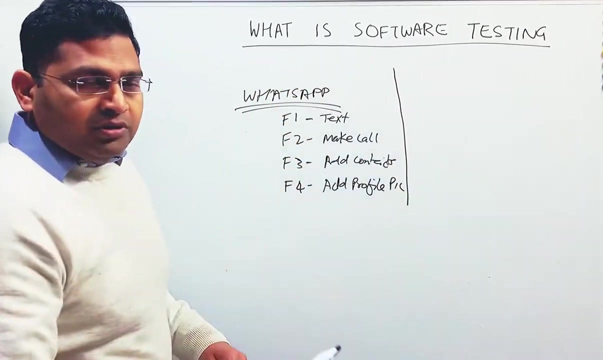 able to text to other person. I should. functionality 3: add contacts right. and then functionality for, say, for example, add profile picture right: add profile pic. so these are some of the functionalities in this particular app. now this is the app. now say, for example, you want to test an e-commerce website. 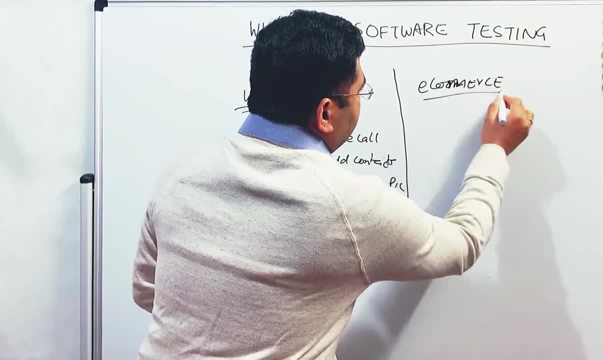 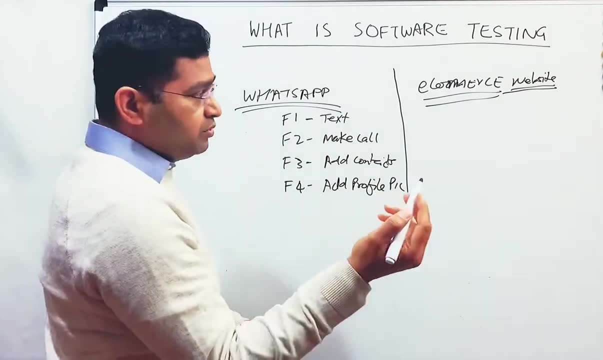 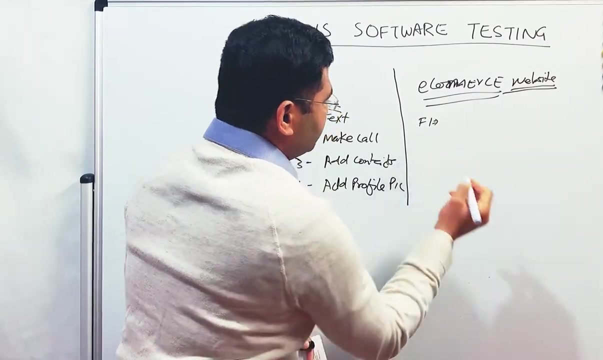 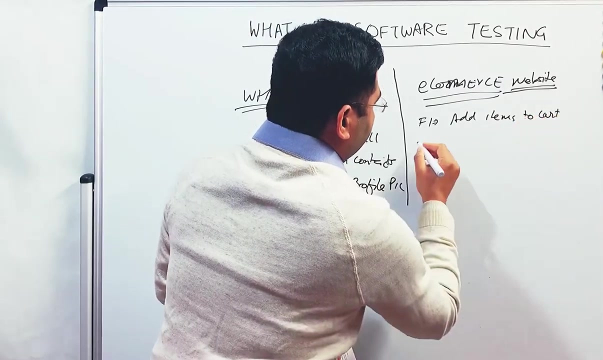 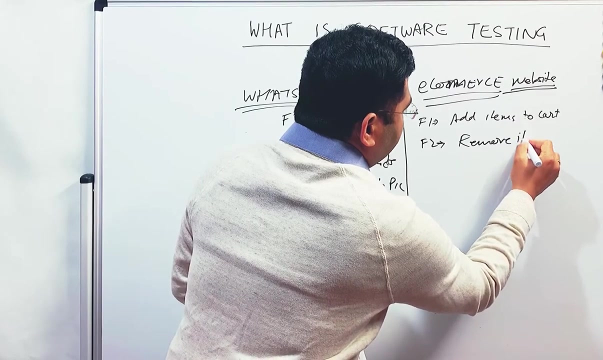 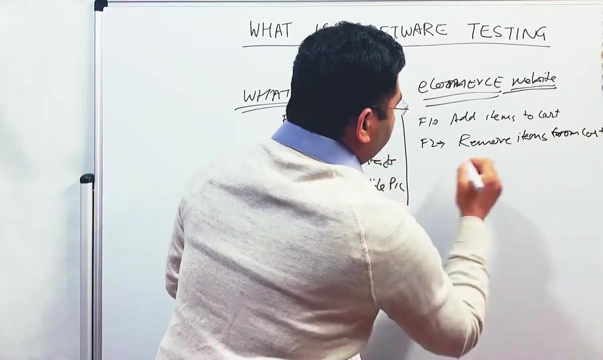 okay, so e-commerce website. so what functionalities that e-commerce website will have? sorry about my handwriting, but this is e-commerce website. so say, for example, functionality 1 is, you know, add items, add items to cart. then functionality to remove items- right, remove items if I want to from cart- okay. so similarly, there'll be, you know like: 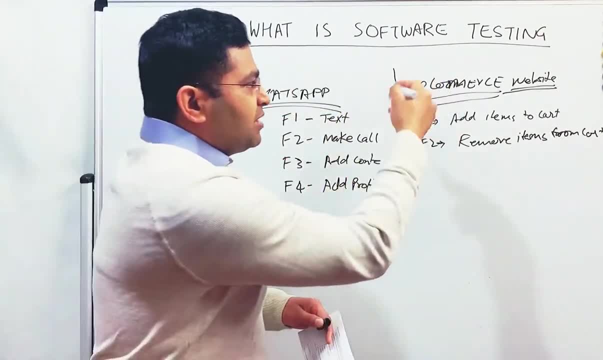 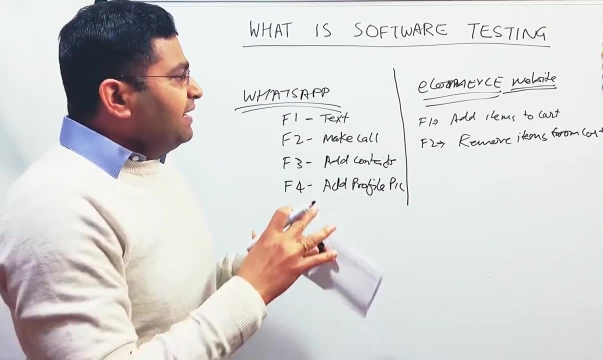 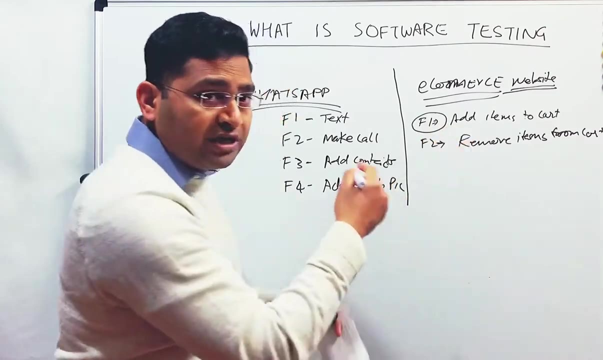 different. so this is the example of the app, this is example of the website which will have, you know, like you know, all a different interfaces, built-in, integration, built-in, and then you, as a tester, will follow a defined process so you have this requirement, this functionality, say, for example, it will have the requirement or it will come as. 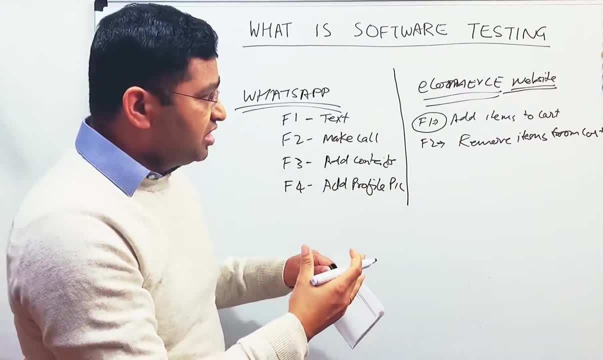 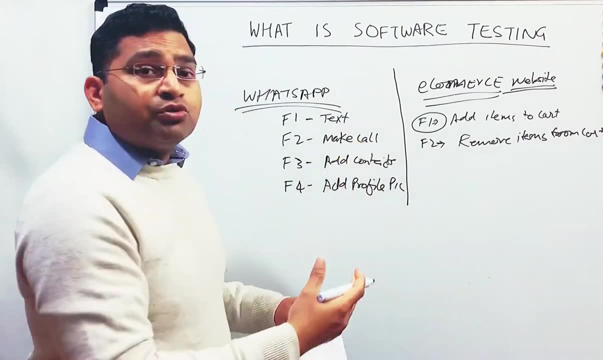 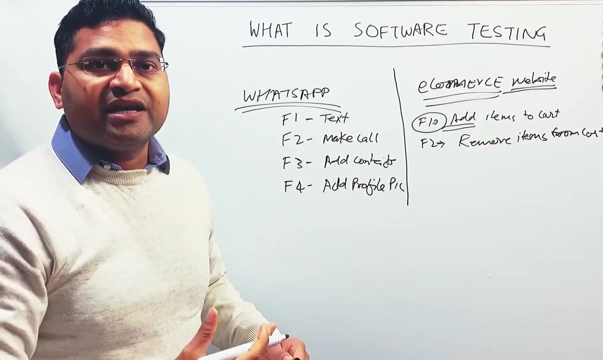 a user story. if you are following scrum methodology or agile approaches, then you will basically go through those user stories and analyze the user stories, write the test cases to ensure that these you know requirements that I've mentioned- say, for example, adding items into the cart. you write test cases. 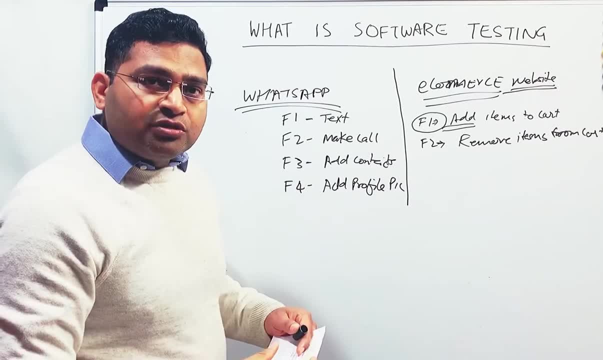 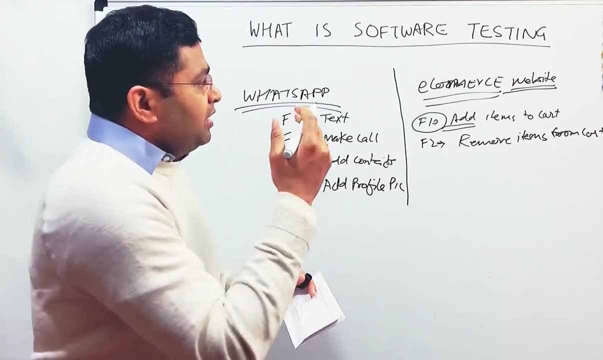 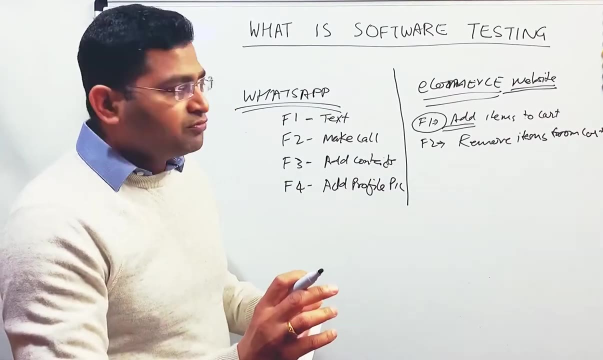 you will then ensure that those test cases actually work as expected. right, so you run the website, you launch the website that is being built and then you will run those test cases. what you will do is you will add the items into the cart. you will try to add the items. you'll try to remove the items from the 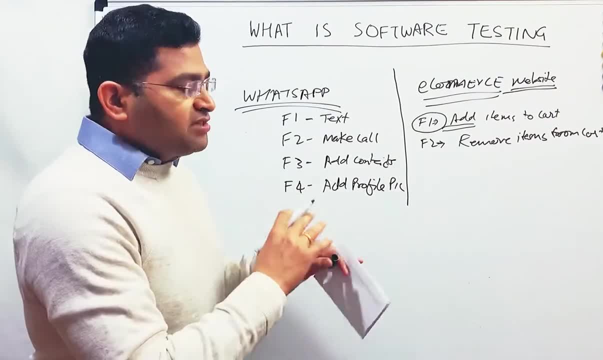 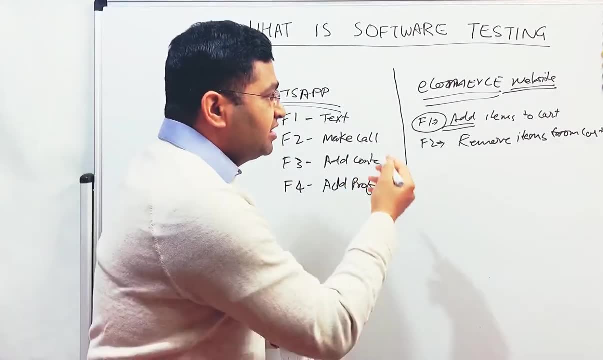 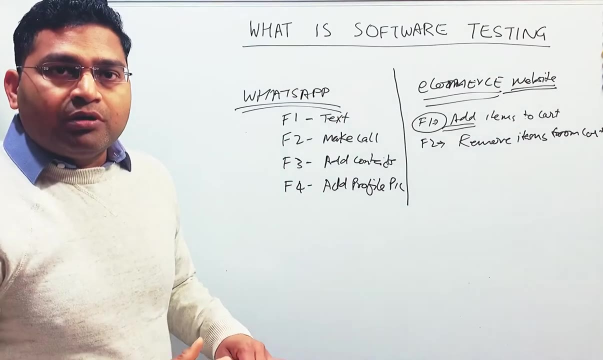 cart and then proceed further. so you'll say, yes, these test cases have passed or these test cases have failed. so if any of the functionality doesn't work as it is defined in the requirement, you will say it has failed, right? so this is the overall example, or with example to 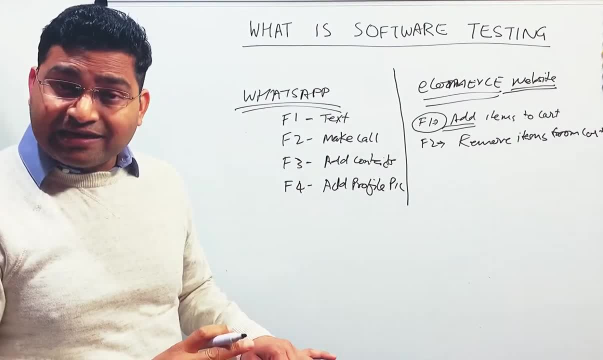 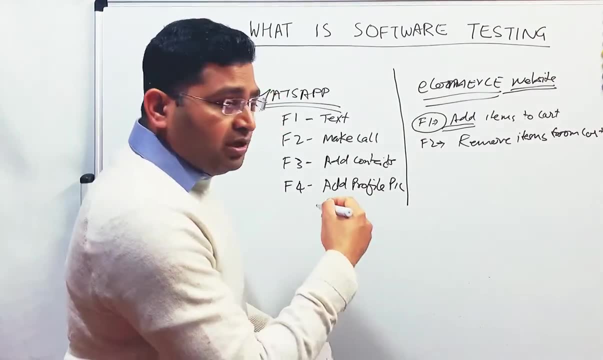 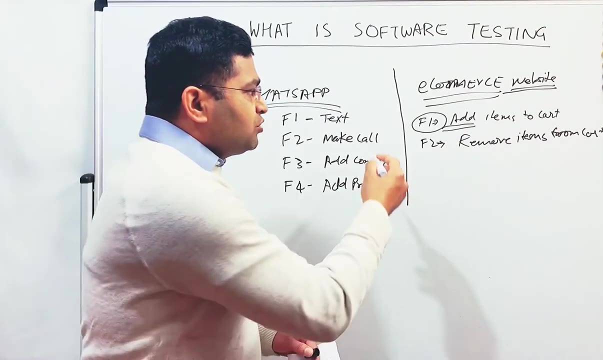 explain you what exactly is software testing. it is not a standalone activity. it is a, you know, a lifecycle and it basically consists of all the static approaches and the dynamic approaches. there are a lot of activities that need to be involved there. say, for example, once you get the requirement, you analyze those requirement as the testing. 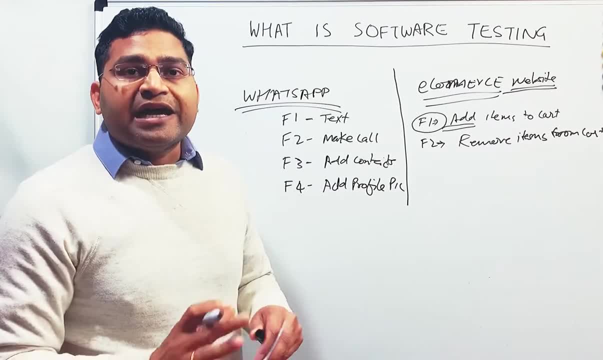 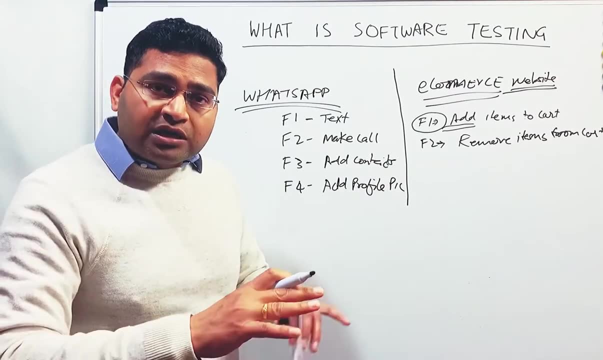 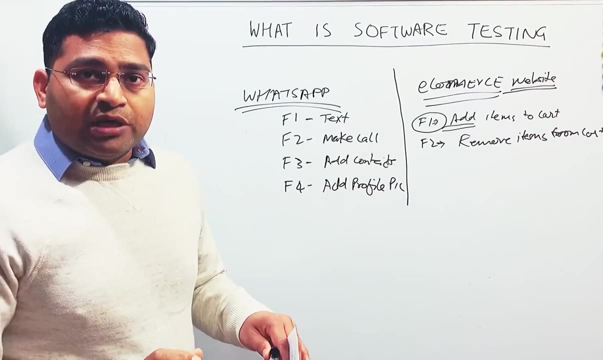 team or tester and see whether there are any gaps into those requirement. so that analysis is the static part. when you design your test cases, you ensure that all the coverage for that particular requirement is there for that particular user story or the requirement all right, so that analysis part is the static part. 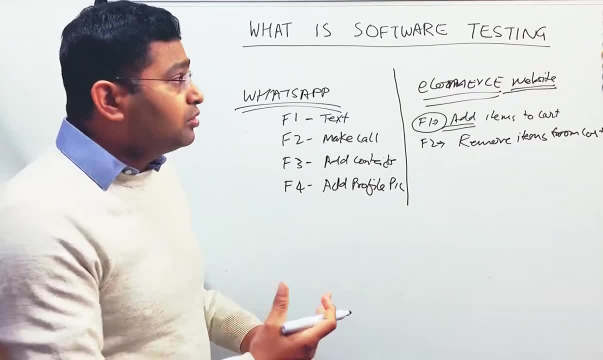 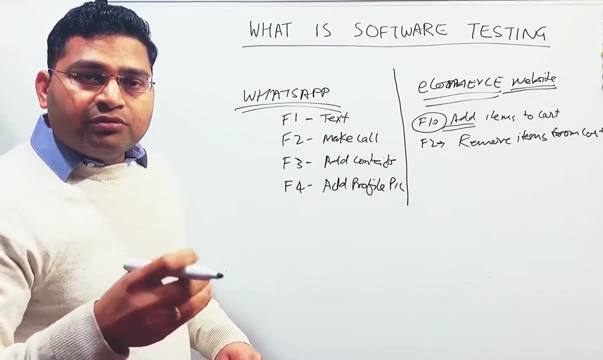 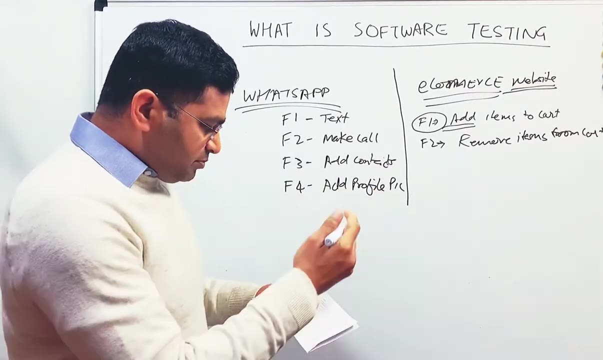 when you execute the code, or when you run the code and actually learn the code and actually launch the website or actually launch the whatsapp on ios or android, and then you know, click on it or test or follow different steps. that's the dynamic part of the software testing, right? so this is basically. you know what exactly software testing that's.